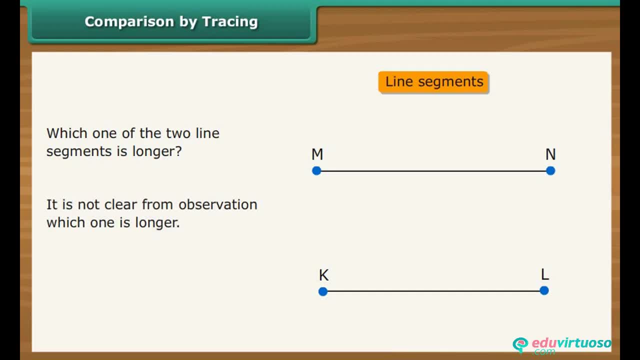 It is not clear from observation which one is longer. Therefore, trace KL on a tracing paper. Place it on MN. It is clear that KL is smaller than MN. Hence MN is the longer line segment. Comparison by measurement: Look at the two line segments AB and CD. Which one of the two line segments MN is shorter than S? Look at the two line segments K, which is shorter than MN. Which one of the two line segments MP and CD B is the longer one? It is not clear from observation which one is longer. 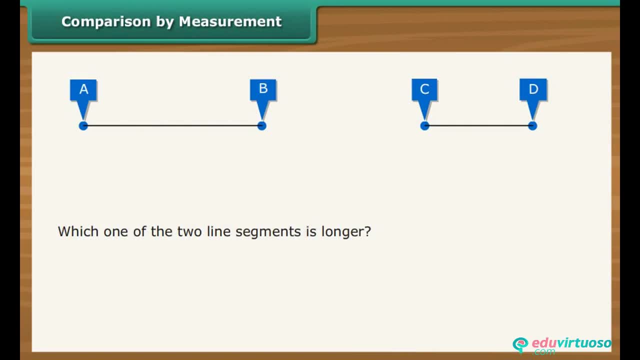 line segments is longer. Let us measure the two line segments with a ruler and decide which one is longer. On one side of the ruler, the measurements are written in inches and on the other side in centimeters. Let us use the centimeter side to measure the line segments. Place the ruler beneath. 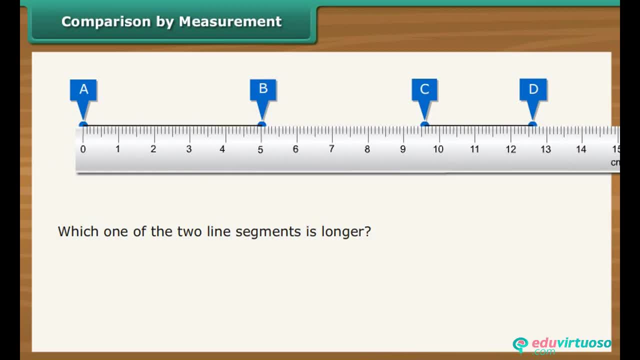 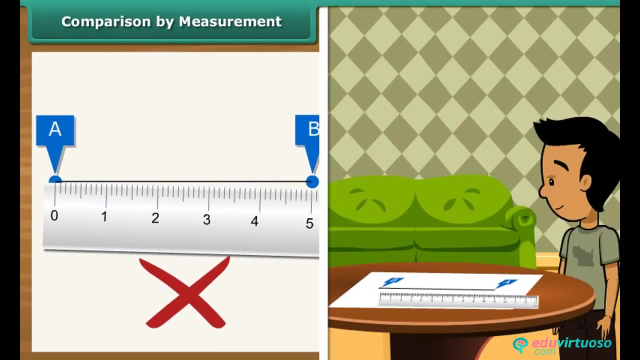 AB such that one end of the ruler is right beneath A Mark. the length of AB. It is 5 centimeter. Repeat the process of CD. The length of CD is 3 centimeter. Therefore AB is longer. Measurements can go wrong if the ruler is not placed right or if the person taking the measurement 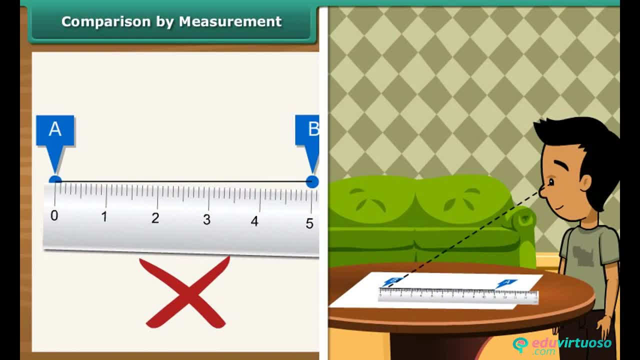 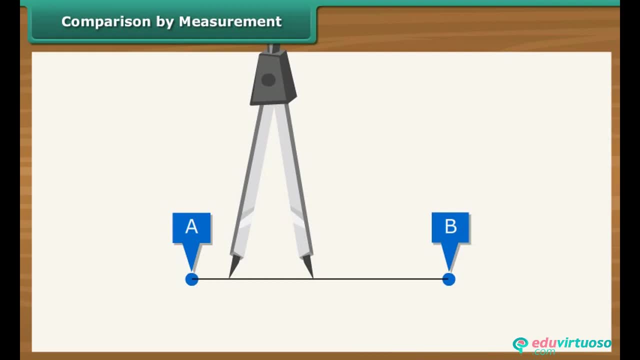 views it from a wrong angle. A better way to measure is to use the divider. Place the divider on AB, such that the sharp end of one arm of the divider is on A and the sharp end of the other arm is on B. Measure AB. Place the divider on the ruler. 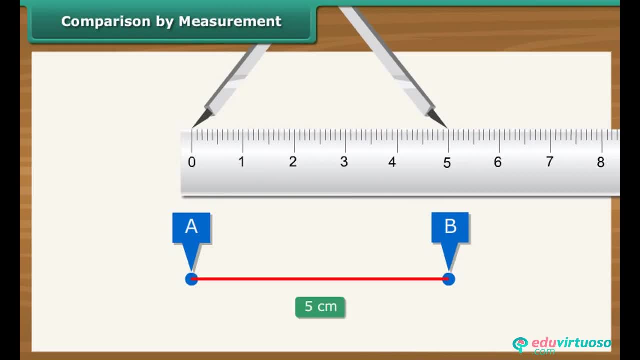 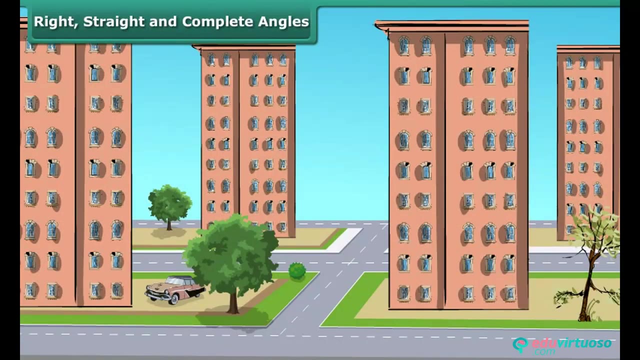 Write down the measurement of AB as 5 centimeter. Now measure CD in the same way. Write down the measurement of CD as 3 centimeter. Therefore, AB is longer. Write straight and complete angles. There are four pockets- A, B, C and D- in a residential locality. 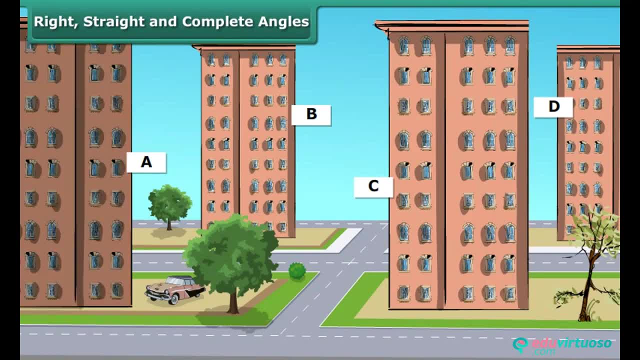 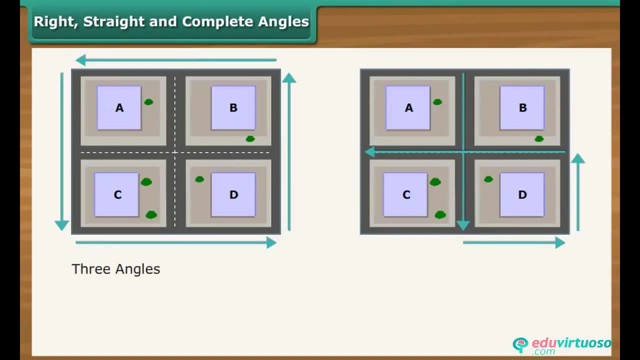 The four pockets are located like this. Rajiv lives in pocket A and is a fitness freak. Every day in the morning he jogs in and around the residential complex. Let us see the two different pockets. There are four different routes he takes. While jogging, Rajiv makes three different angles. 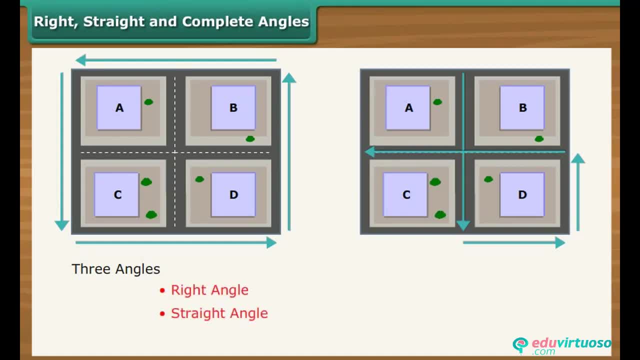 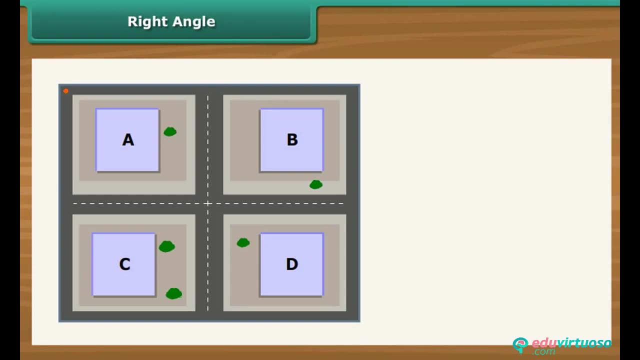 They are: right angle, straight angle, complete angle. Let us look at each angle in detail. Right angle: Let us look at the first route that Rajiv takes for jogging. He jogs from pocket A to pocket C, turns left, jogs to pocket D. 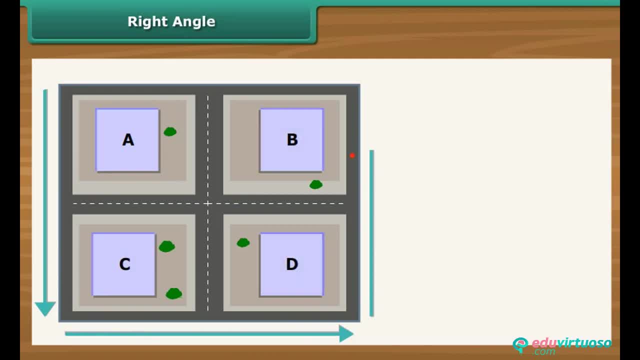 turns left once more and jogs back to pocket A. Every time Rajiv turns left he makes a right angle of 90 degree. Thus in one full round he makes four right angles: Straight angle. Let us look at the second route that Rajiv takes for jogging. 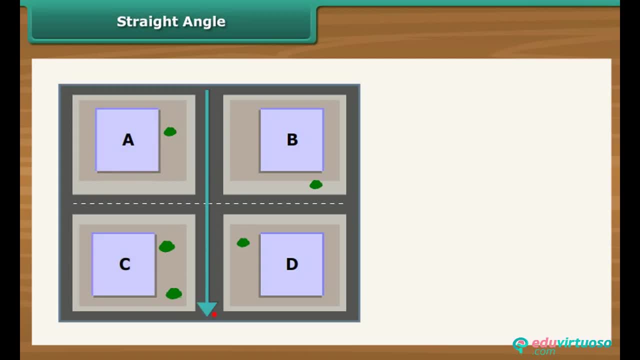 He jogs from pocket A to pocket C, turns left, jogs to pocket D, turns left again, jogs half way towards pocket B, turns left once more, jogs to pocket A. When Rajiv jogs from pocket A to pocket C, he covers two right angles. 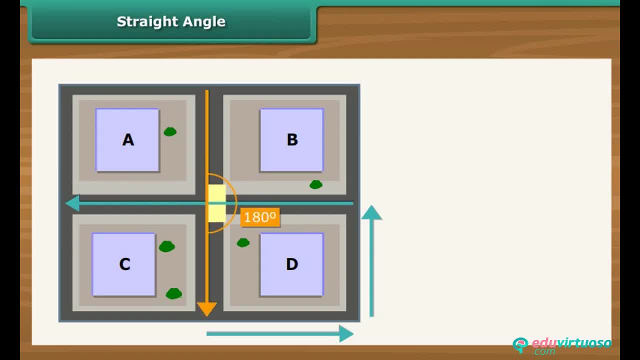 In other words, he covers a straight angle of 180 degrees. Rajiv covers another straight angle in this jogging route. Can you identify it? Yes, When he jogs from pocket B to pocket A, he covers another straight angle, Complete angle. Let us take a second look at the first route that Rajiv takes for jogging. 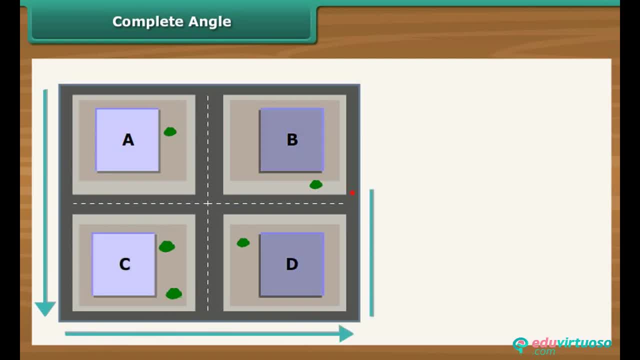 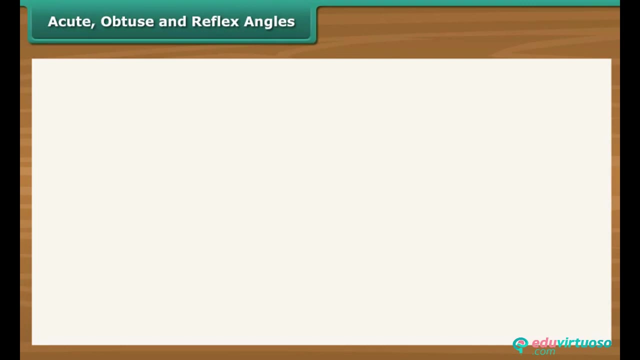 He jogs from pocket A to C, to D to B and then back to A. In a single round he covers four right angles. In other words, he covers a complete angle of 360 degrees: Acute, obtuse and reflex angles. There are three more angles. They are: 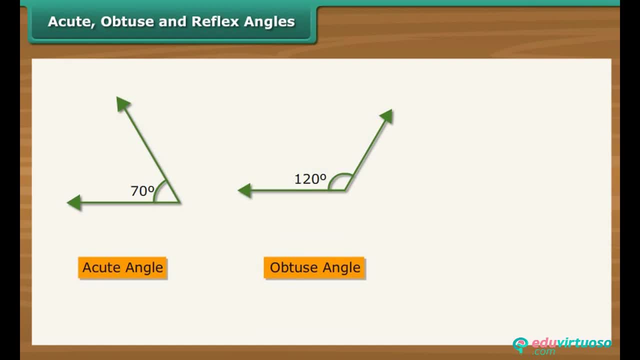 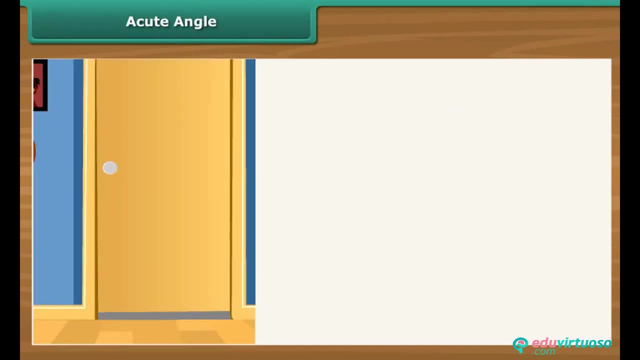 acute angle, obtuse angle, reflex angle. Let us look at them one by one. Acute angle: Look at this picture of an open door. Can you identify the angle that it makes with the ground? Yes, 90 degree. Now shut the door slowly. 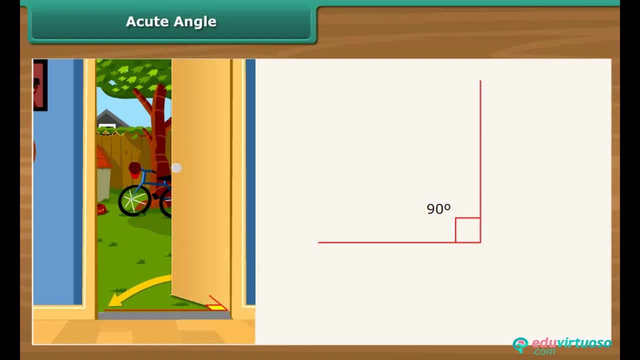 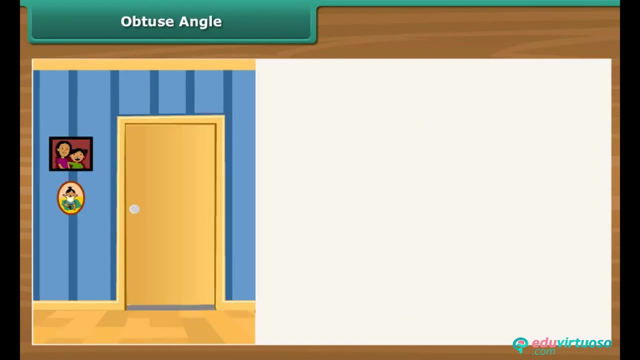 Can you identify the angle that it now makes with the ground? You are right: Less than 90 degree. Angles that measure less than 90 degree are called acute angles, Obtuse angle. Let us go back to the picture of open door. 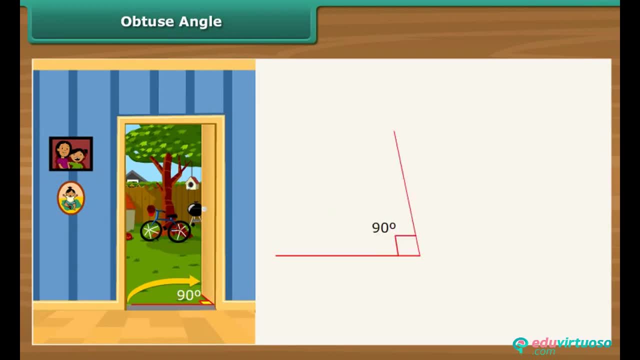 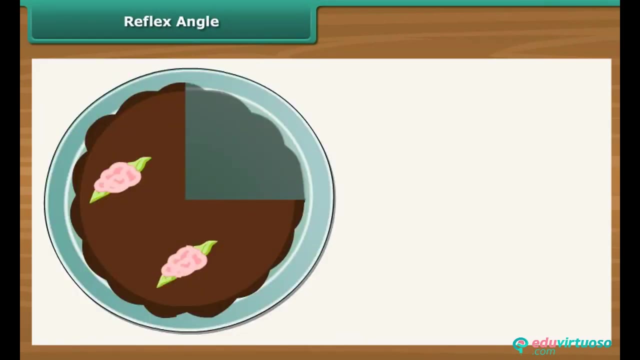 What do you think will happen if you push the door further to the right? The measure of the angle will exceed 90 degrees. Angles that measure more than 90 degree are called obtuse angle- Reflex angle. Look at this cake. One-fourth of it has been sliced out. 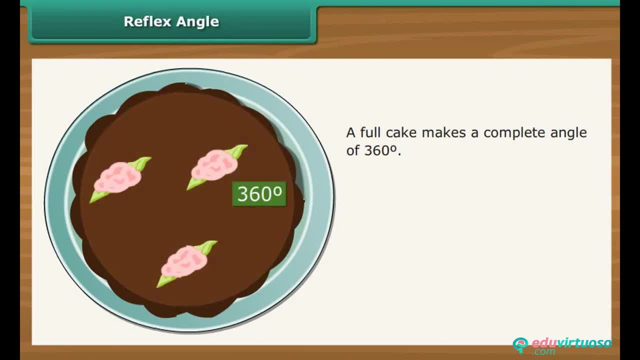 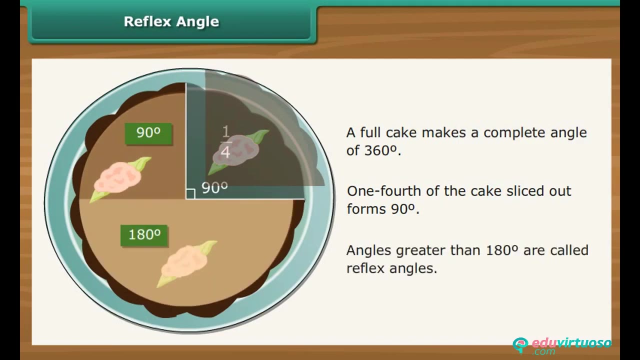 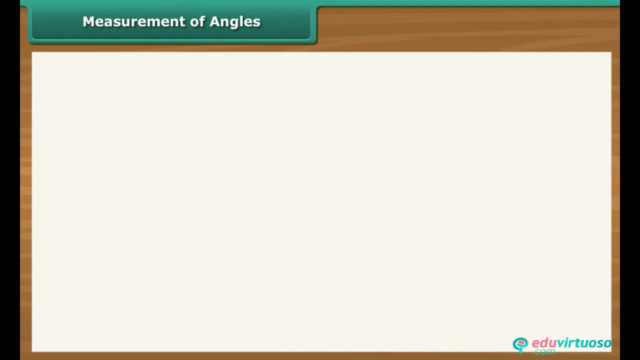 A full cake makes a complete angle of 360 degrees. One-fourth of the cake sliced out forms 90 degree. The cake that remains forms 270 degree. Angles greater than 180 degree are called reflex angles- Measurement of angles. Let us now learn to measure angles with a protractor. 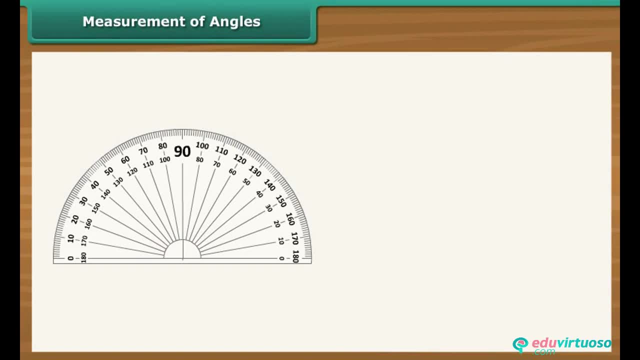 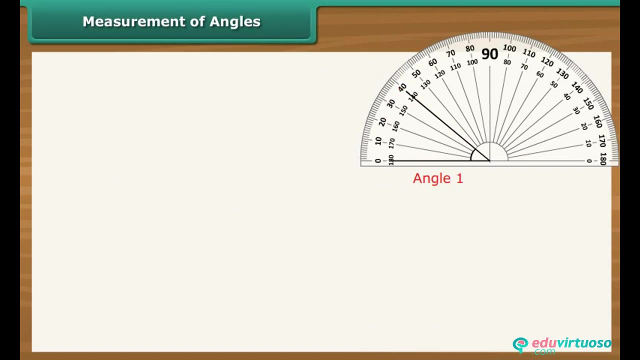 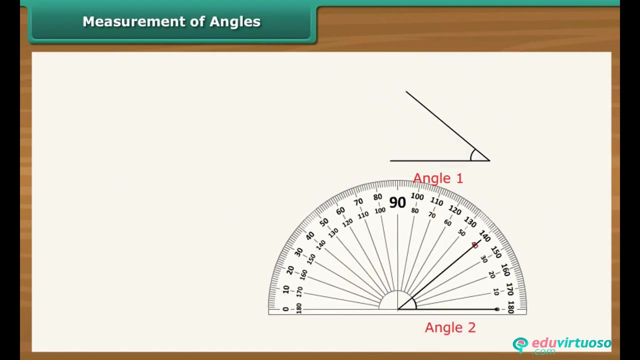 Protractor is a semicircular geometric instrument with markings from 0 to 180.. These markings represent degrees. The outer markings are used to measure an angle. The inner markings are used to measure an angle whose vertex is formed on the left. The inner markings are used to measure an angle whose vertex is formed on the right. 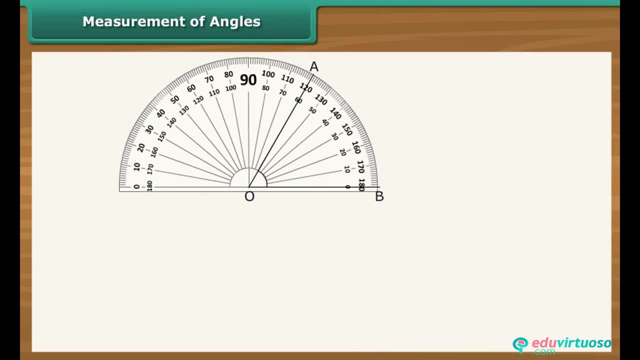 Measure angle AOB with the help of the protractor. Place the protractor on ray OB. Ensure that the horizontal line at the bottom of the protractor coincides with OB and its midpoint rests on vertex O. Check the inner marking that coincides with ray OA. 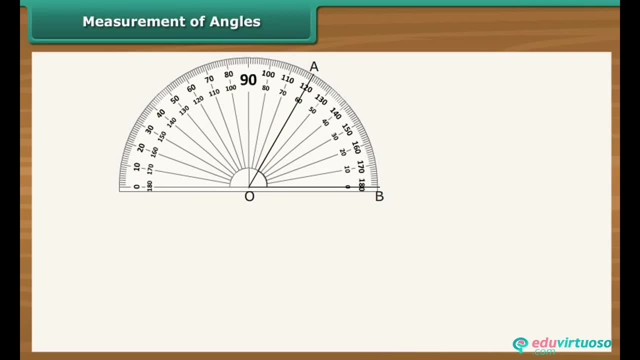 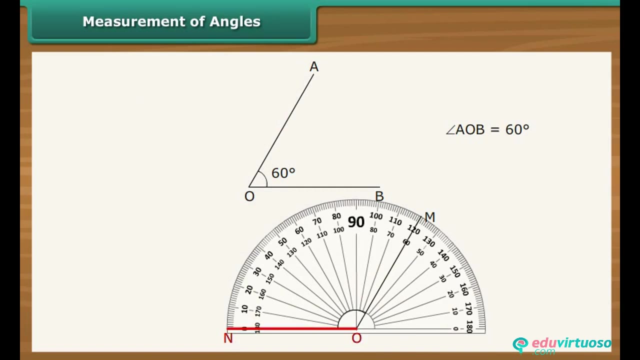 It is 60. Therefore, the measure of angle AOB is 60 degree. Measure angle MON. with the help of the protractor, Place the protractor on ray OM, Ensure that the horizontal line at the bottom of the protractor coincides with ON and its midpoint rests on vertex O. 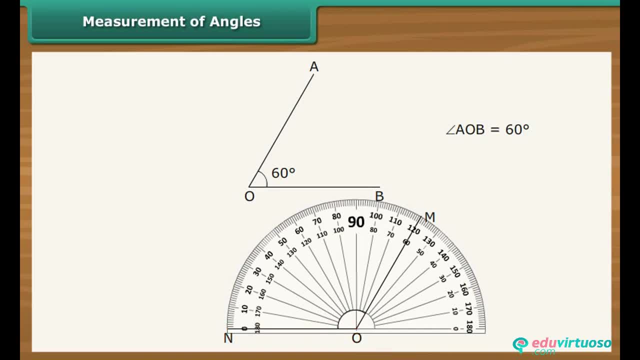 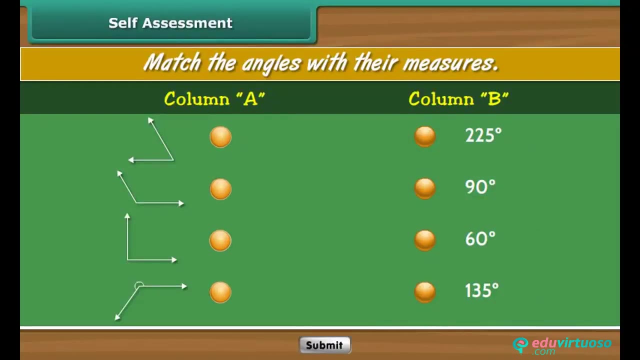 Check the outer marking that coincides with ray OM. It is 120.. Therefore, the measure of angle MON is 120 degree. Self-assessment: Match the angles with their measures. Measure angle AOB with the help of the protractor. Place the protractor on ray OM. 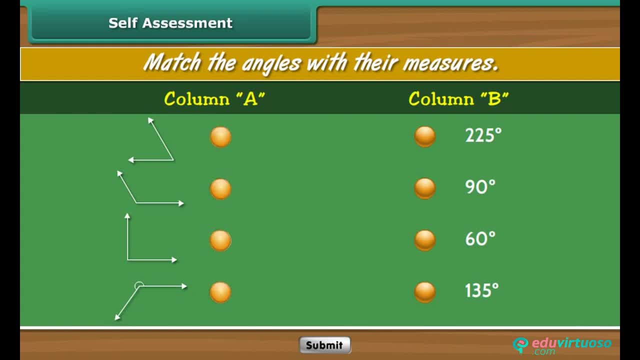 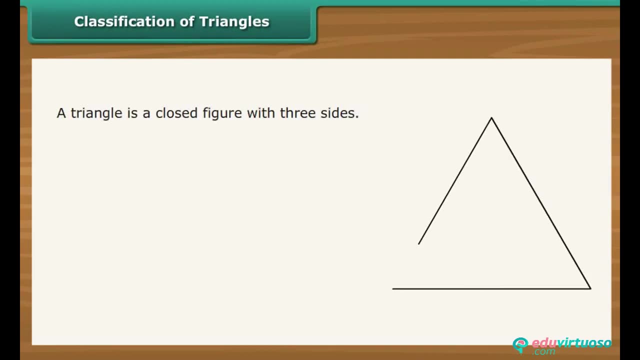 Ensure that the horizontal line at the bottom of the protractor is 60 degree. Ensure that the horizontal line at the bottom of the protractor is 60 degree. Classification of triangles. A triangle is a closed figure with three sides. We can classify all triangles on the basis of their sides. 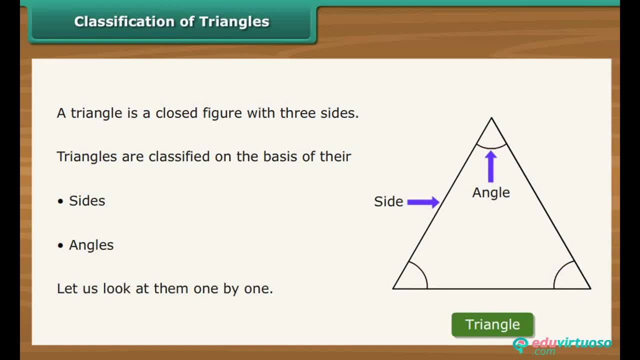 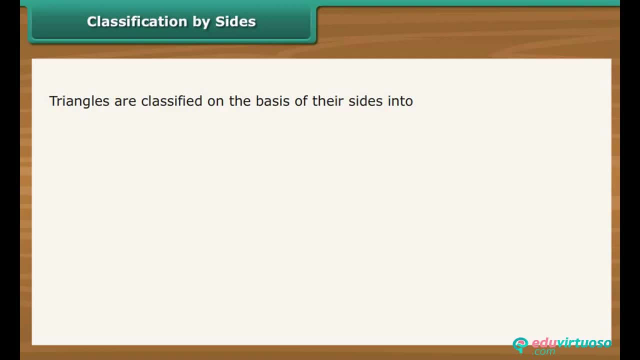 Let us look at them one by one. Classification by sides. Triangles are classified on the basis of their sides, into equilateral triangles, isosceles triangles, scalene triangles. Triangles in which all the three sides are equal are known as equilateral triangles. 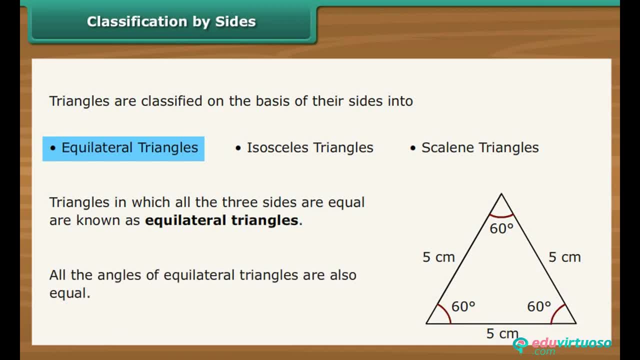 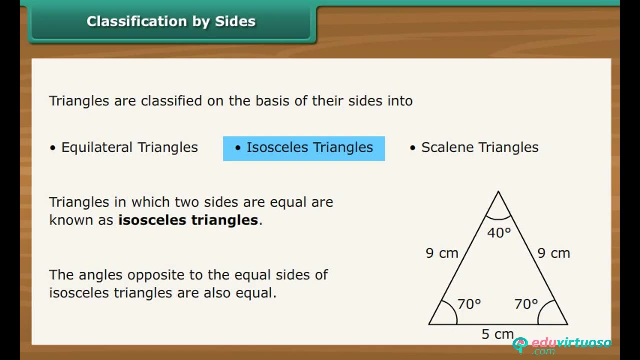 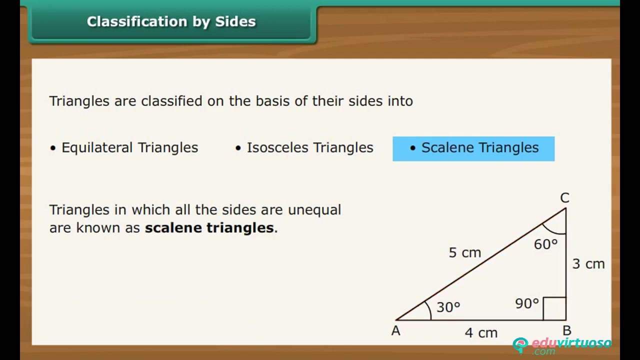 All the angles of equilateral triangles are also equal. Triangles in which two sides are equal are known as isosceles triangles. The angles opposite to the equal sides of isosceles triangles are also equal. Triangles in which all the sides are unequal are known as scalene triangles. 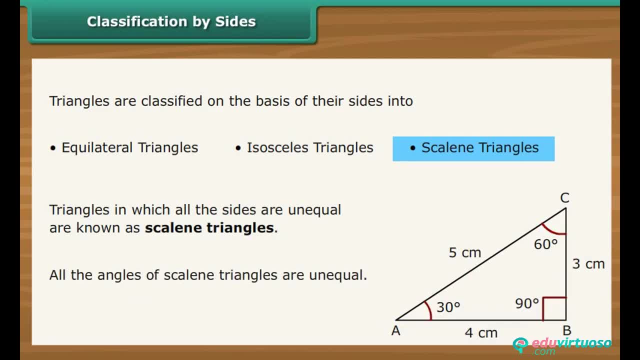 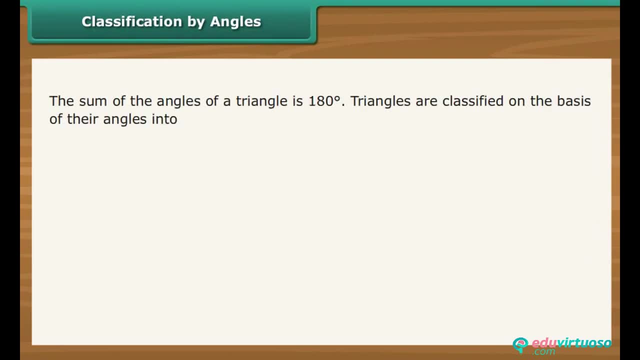 All the angles of scalene triangles are unequal. Classification by angles: The sum of the angles of a triangle is 180 degree. Triangles are classified on the basis of their angles into acute angled triangles, right angled triangles, obtuse angled triangles, Triangles in which all the three angles measure less than the other angles. 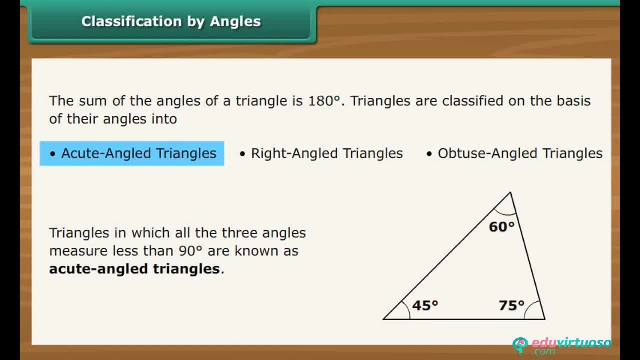 less than 90 degree are known as acute angled triangles. Triangles in which any one angle measures exactly 90 degree are known as right angled triangles. Triangles in which any one angle measures more than 90 degree are known as obtuse angled triangles. 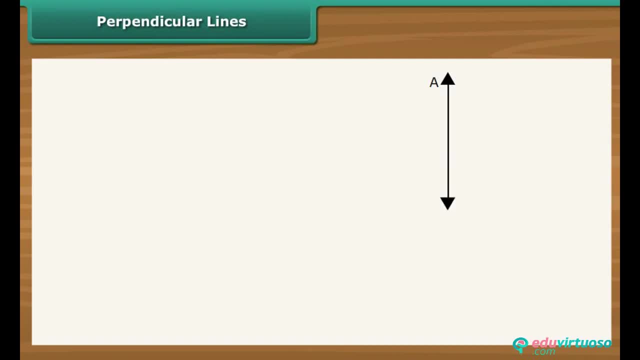 Perpendicular lines. Look at these two lines: A, B, intersects C, D. The point of intersection of the two lines is O. The four angles formed at the point of intersection are 90 degree each. Therefore, the two lines are said to be perpendicular to each other. 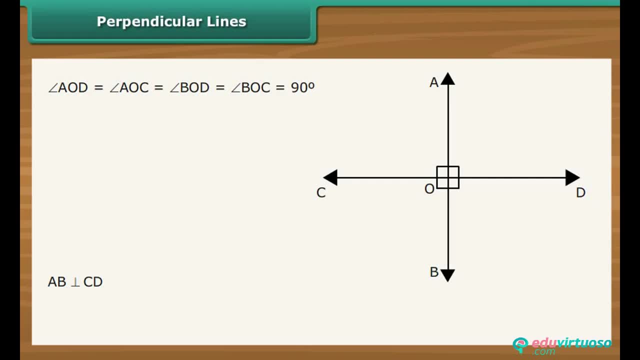 If O is also the midpoint of C D, then A B bisects C D because it divides C D into two equal halves. Such a line which intersects another line at the point of intersection of C D, such a line which intersects another line at right angles. 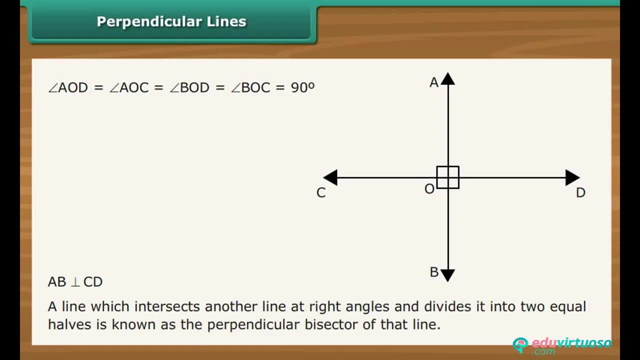 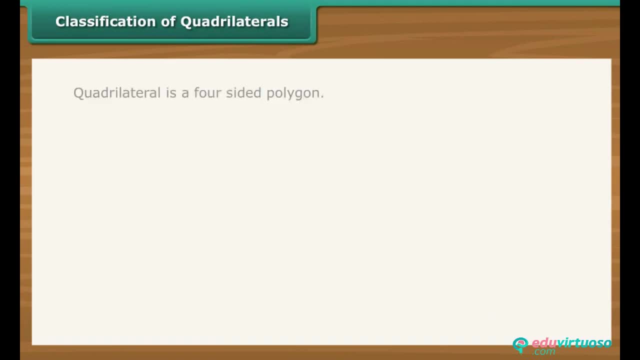 and divides it into two equal halves is known as the perpendicular bisector of that line. Classification of Quadrilaterals. Quadrilateral is a four-sided polygon. Quadrilaterals are classified as rectangle, square, parallelogram, rhombus trapezium. Let's learn the properties of each. 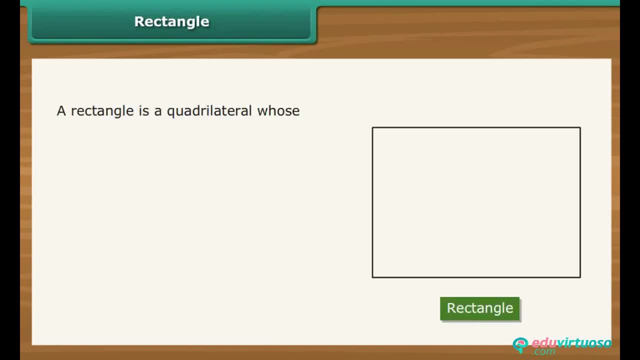 Rectangle. A rectangle is a quadrilateral whose opposite sides are equal and parallel, whose four angles are equal, whose each angle measures 90 degree, whose diagonals are equal and perpendicular to each other. Square- A square is a quadrilateral whose four sides are equal. 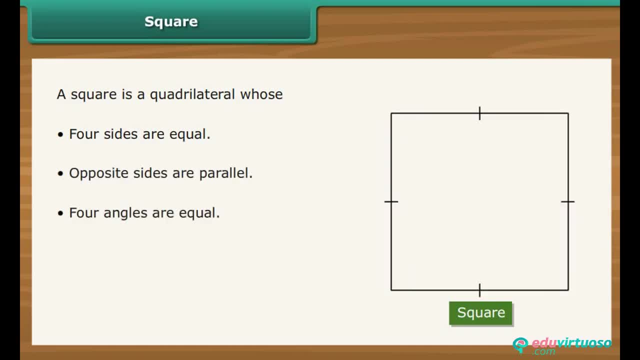 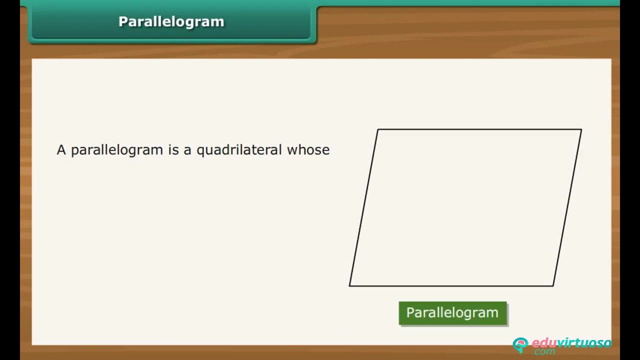 whose opposite sides are parallel, whose four angles are equal, whose each angle measures 90 degree, whose diagonals are equal and perpendicular to each other. Parallelogram- A parallelogram is a quadrilateral whose opposite sides are equal and parallel. 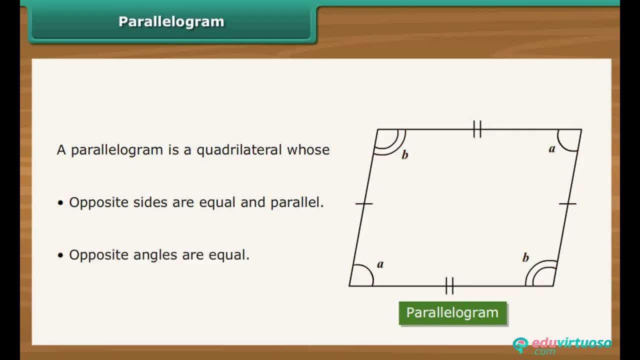 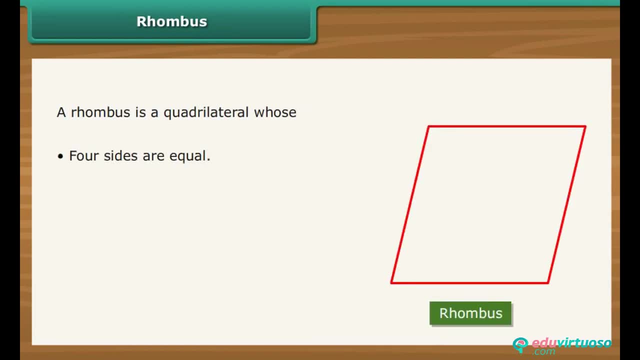 whose opposite angles are equal. Rhombus- Rhombus is a quadrilateral whose four sides are equal and parallel, whose opposite sides are parallel, whose four angles are equal and perpendicular to each other. Quadrilateral: A sansquare is a quadrilateral whose opposite sides are parallel and parallel. 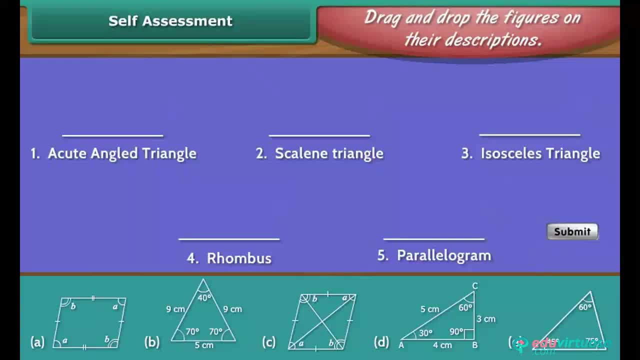 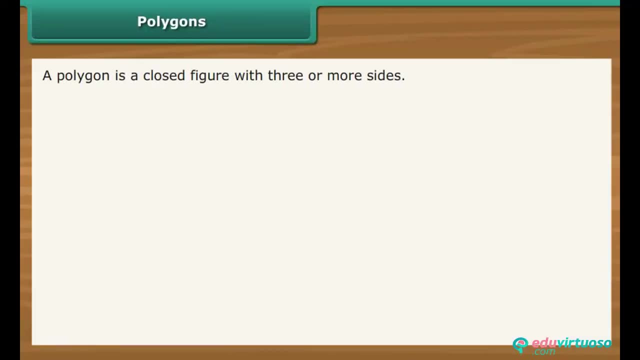 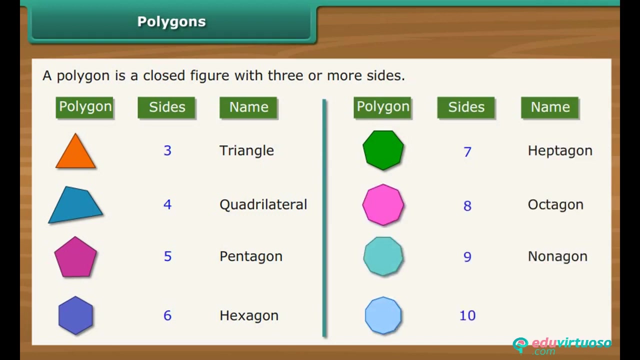 Self-assessment. Let us know how much you have learned. Drag and drop the figures on their descriptions: Polygons: A polygon is a closed figure with three or more sides. Here are some polygons. Let us count their sides and name them. Three-dimensional shapes have depth. 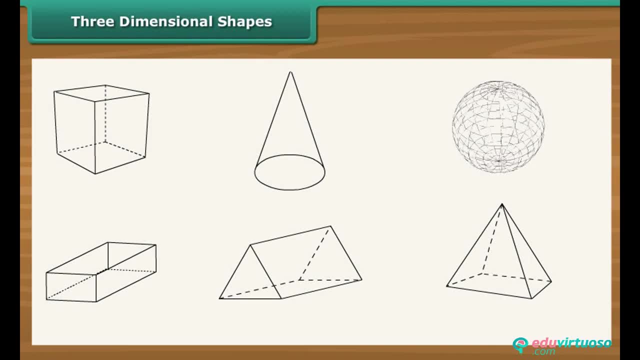 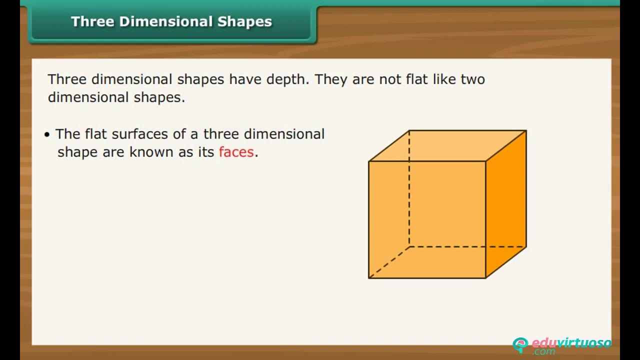 They are not flat like two-dimensional shapes. Examples of three-dimensional shapes are cube, cone sphere, cuboid, prism, pyramid, etc. The flat surfaces of a three-dimensional shape are known as its faces. The points where two faces meet are known as edges. 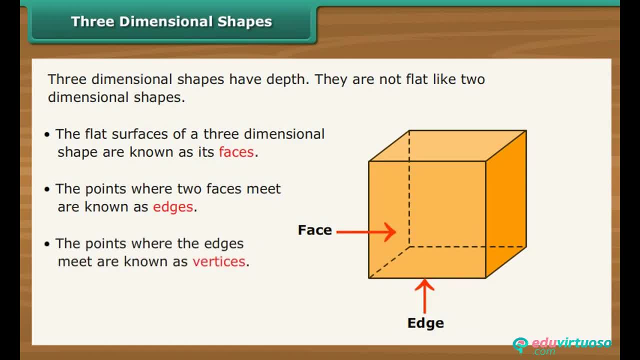 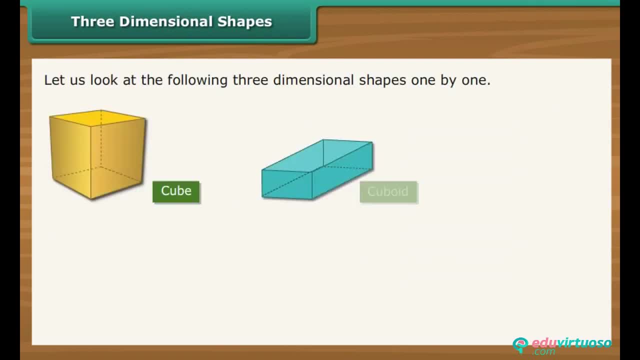 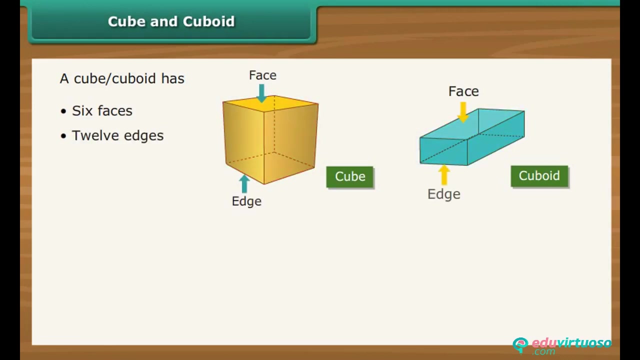 The points where the edges meet are known as vertices. Let us look at the following three-dimensional shapes: Cube and cuboid, triangular, prism, square pyramid. Cube and cuboid. A cube cuboid has six faces, twelve edges, eight vertices. 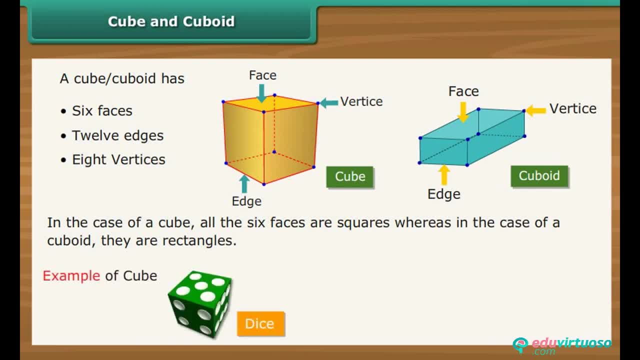 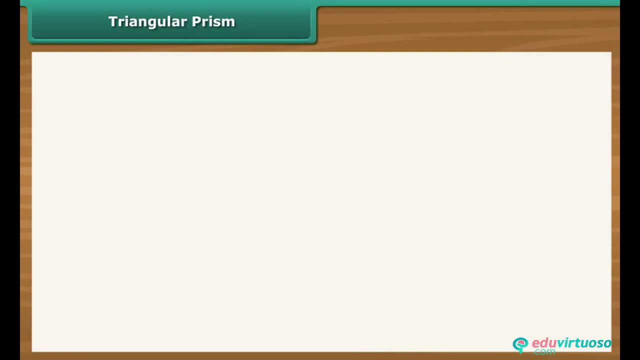 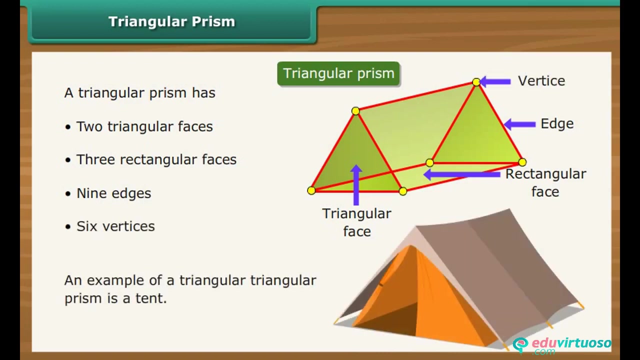 An example of a cube is a dice. An example of a cuboid is a book. Triangular prism. A triangular prism has two triangular faces, three rectangular faces, nine edges, six vertices. An example of a triangular prism is a tent. 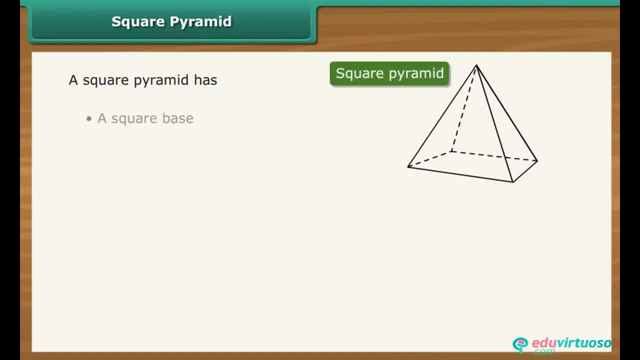 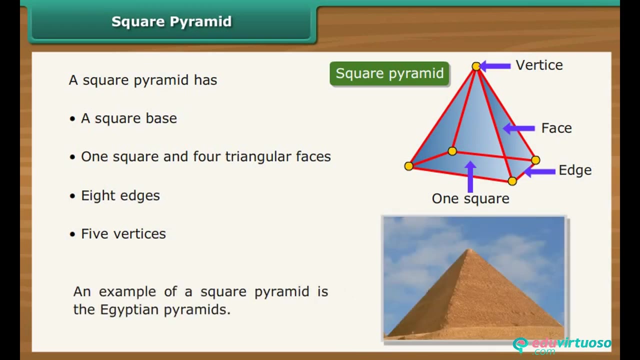 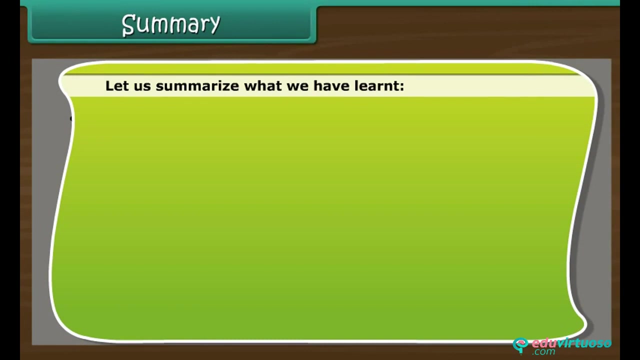 Square pyramid. A square pyramid has a square base, one square and four triangular faces, eight edges, five vertices. An example of a square pyramid is the Egyptian pyramids. Summary. Let us summarize what we have learned. Angles are classified as acute, right, obtuse, straight.